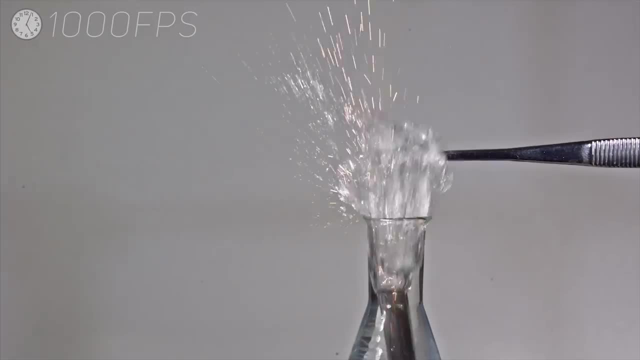 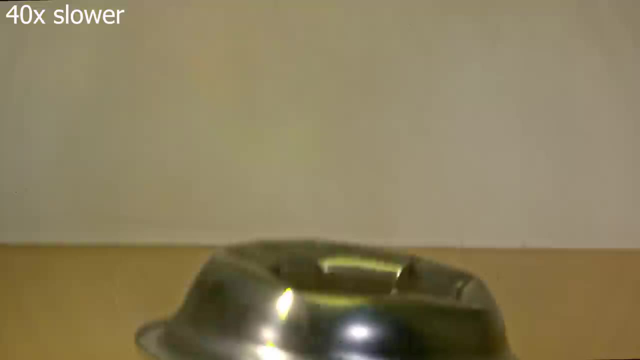 Hey guys, In my videos you have seen a lot of different explosive reactions, but remember that time I showed you the decaborane and nitric acid reaction. It caused a massive explosion easily punching through a steel plate. This particular reaction stands out as the most. 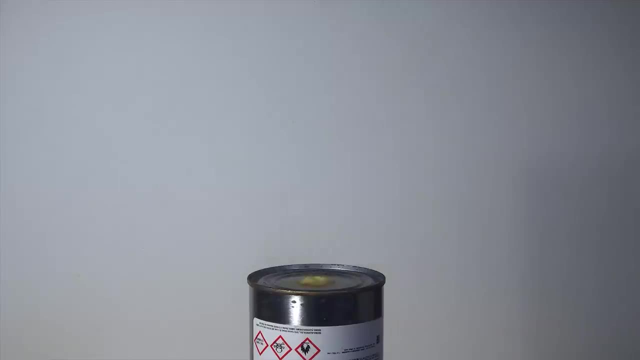 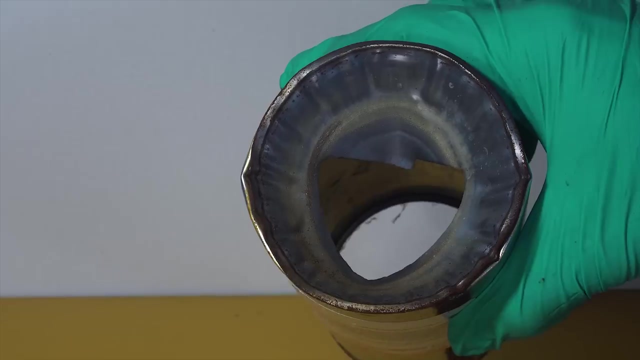 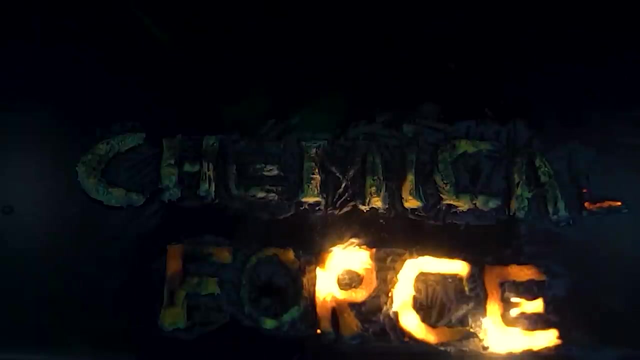 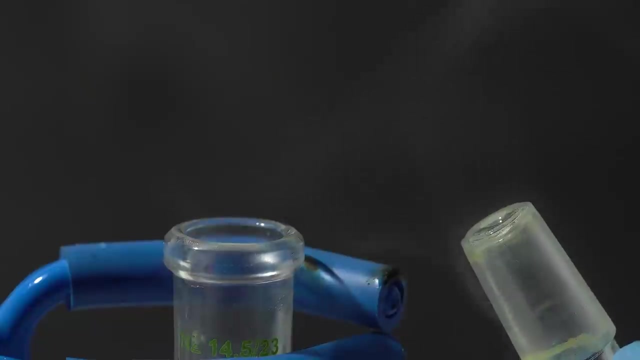 destructive I've ever seen when combining two known explosive components. I haven't found any documentation and articles on it, so, as a discoverer, I call it chemical force reaction. So the first component of this destructive chemical reaction is fuming nitric acid containing. 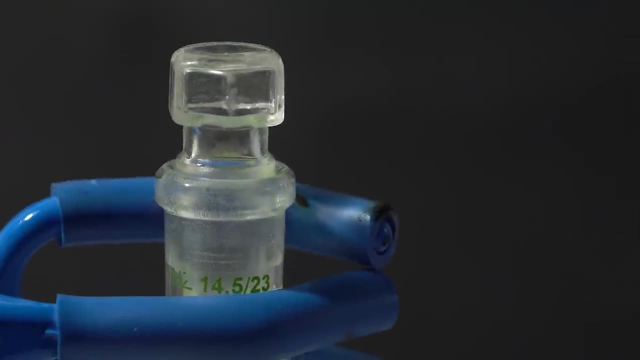 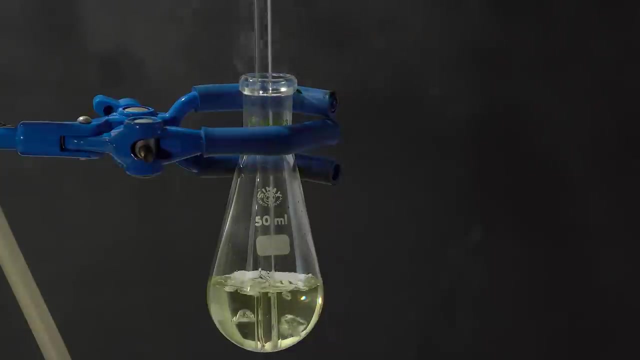 a minimal amount of water. Due to a nitrogen dioxide dissolved in it, it has a yellow-orange tint, so I'll pass a current of dry ozone through acid to make a transparent liquid. Now it's crystal clear nitric acid, as it should be. This liquid can very quickly ignite many organic 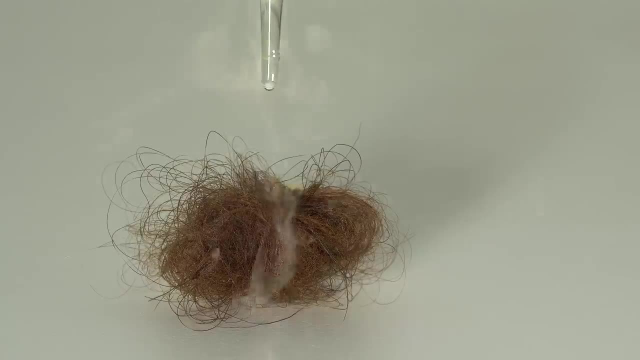 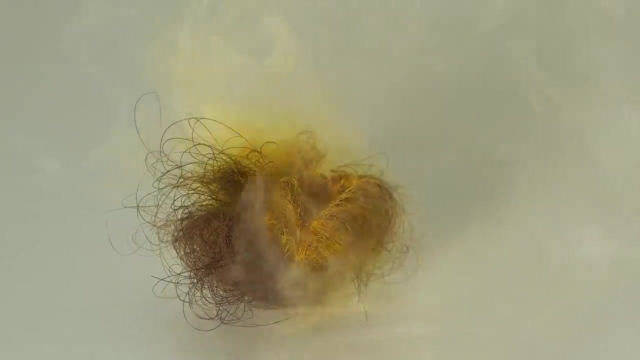 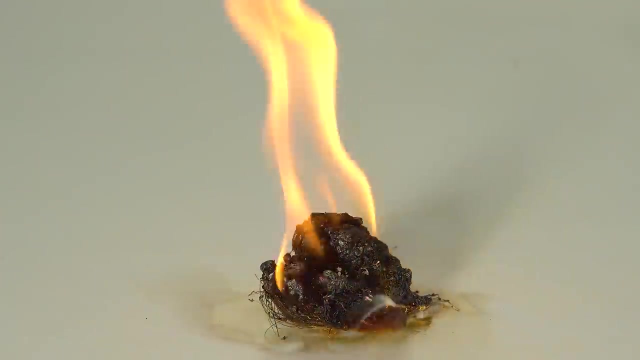 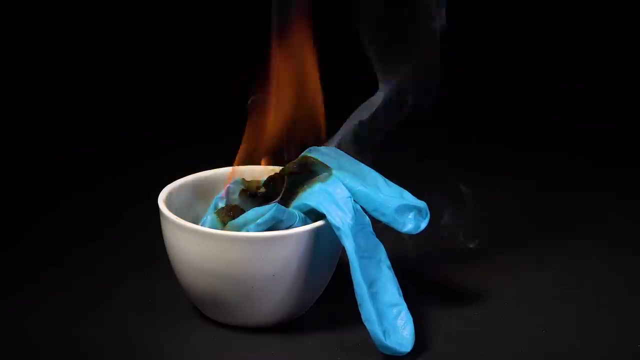 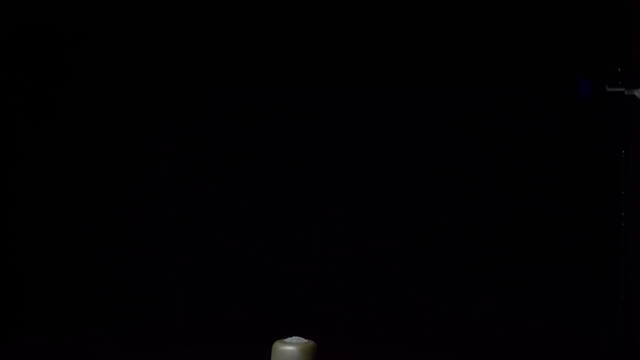 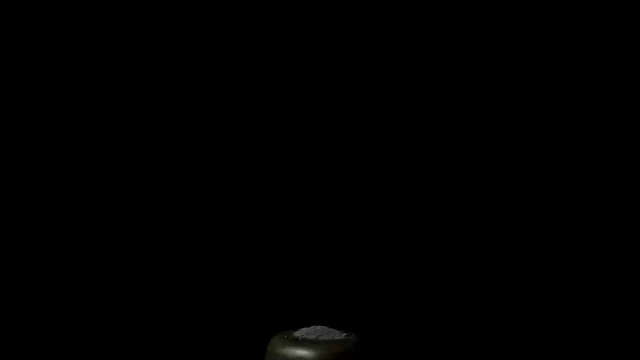 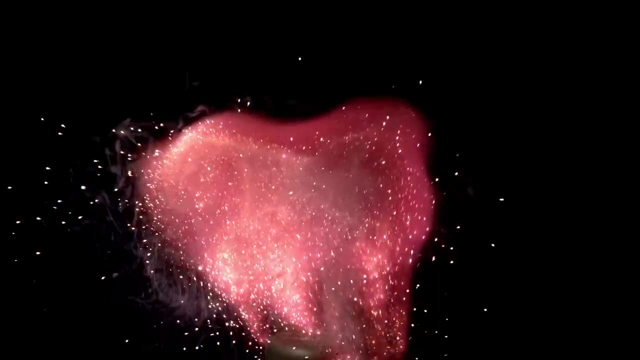 materials such as my hair or ordinary laboratory gloves. I here, I'm150% sure it won'tkö. And this is a just a beautiful reaction with lithium, aluminum hydride, Cmmm, Music, Chmmmmmm. What is aluminum nitric? 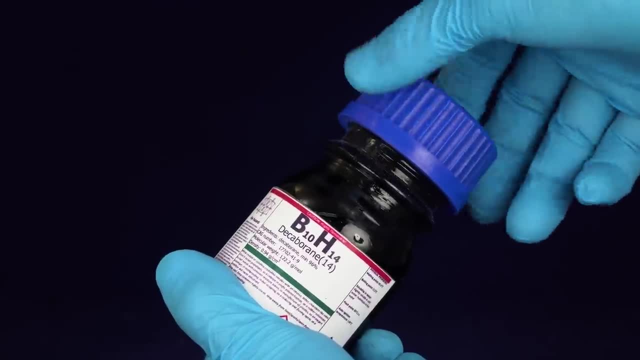 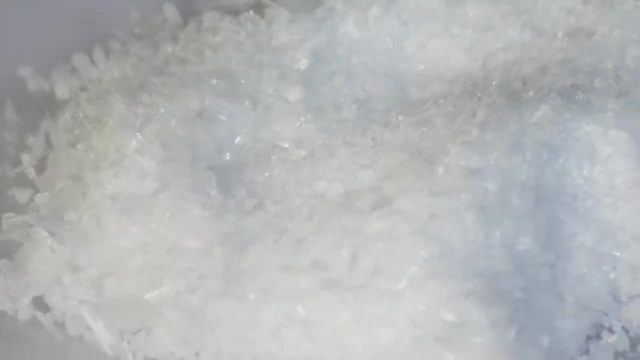 This component is boron hydride decaborane. Let's try it with the reaction mechanism decaborane. This white powder, stores enormous energy and in its individual state, like nitric acid, it's absolutely not explosive, but is a highly flammable reagent. 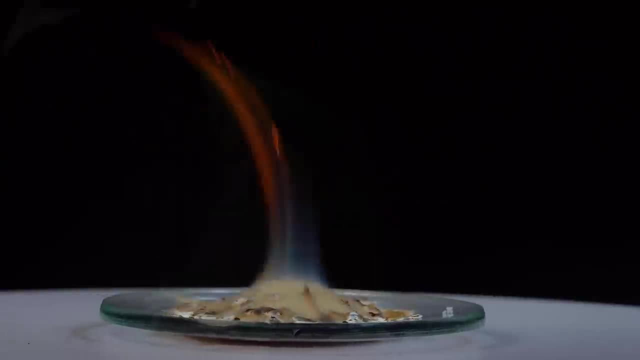 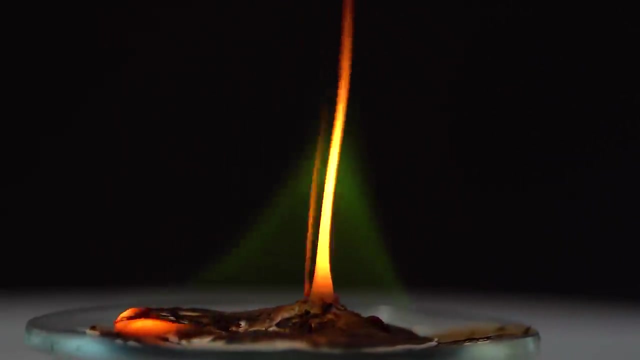 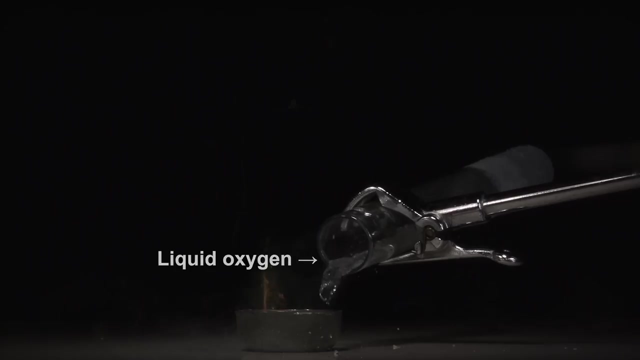 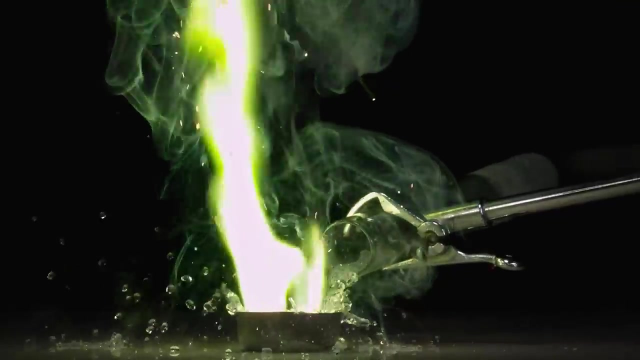 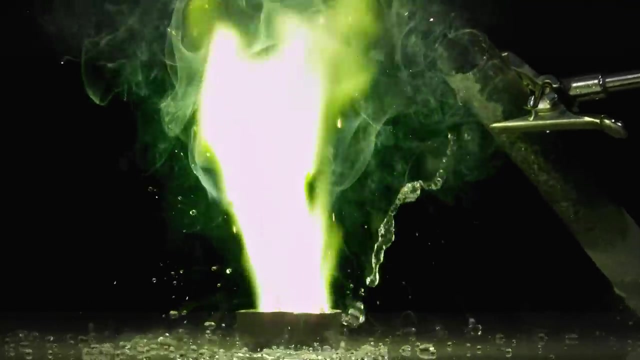 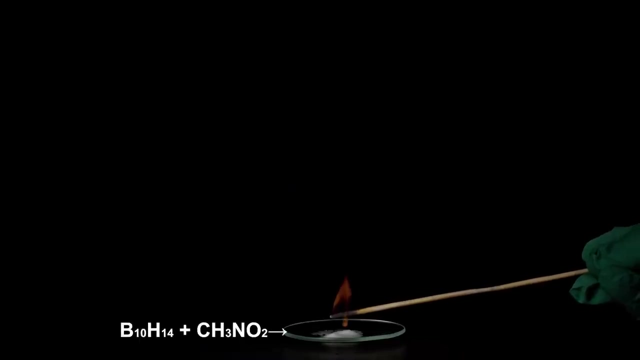 Since this substance contains boron, during combustion we can observe the green color of the flame. We can observe a brighter green color if we add liquid oxygen to the burning- decaborane. The combustion of a mixture of decaborane and nitromethane looks even more impressive. 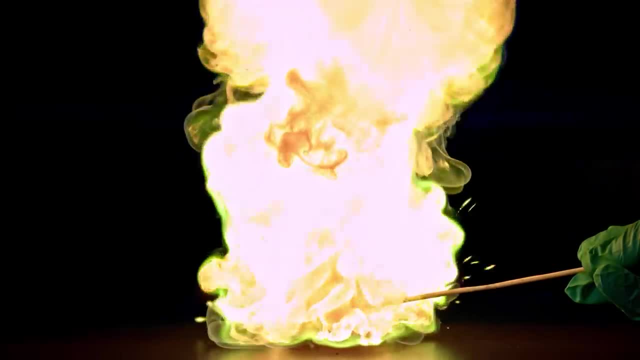 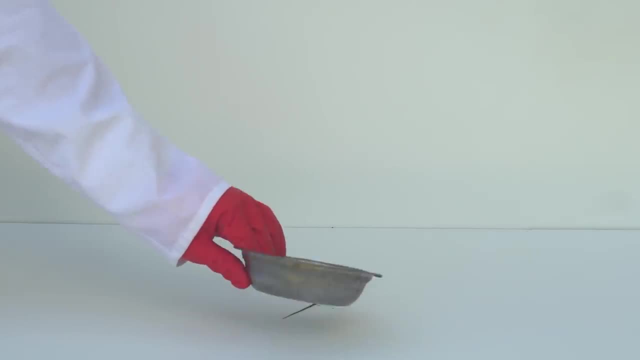 Now let's go outside the lab and see what a mixture of humenitric acid and decaborane is capable of. So the first reaction will be on the surface of a steel bowl When mixing these components. the reaction does not occur immediately, it has a rather 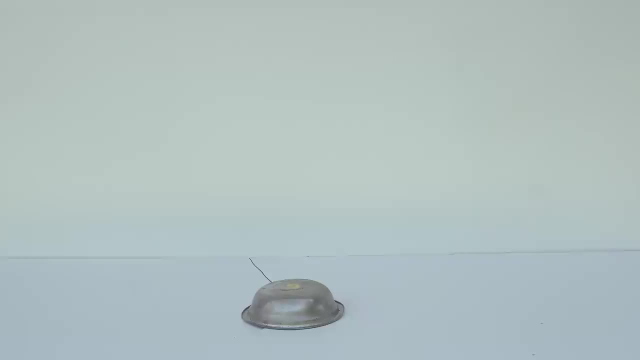 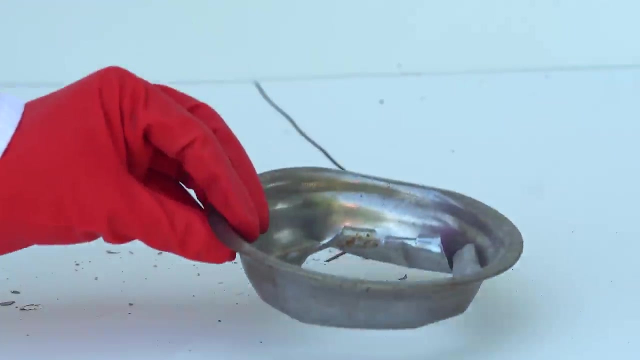 long induction period in order to run away as far as possible. Let's go. So, guys, how do you like such destructive power? Be sure to share your impressions in the comments. You may have noticed cracks on my table for this experiment. 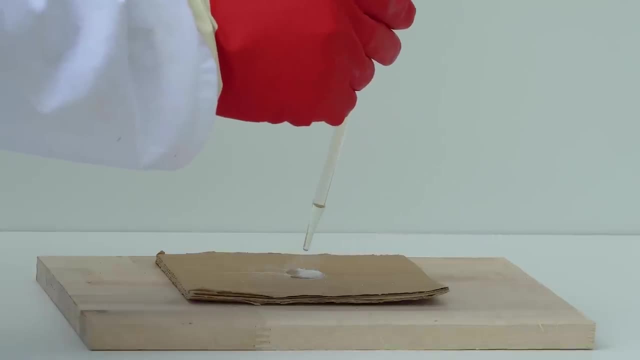 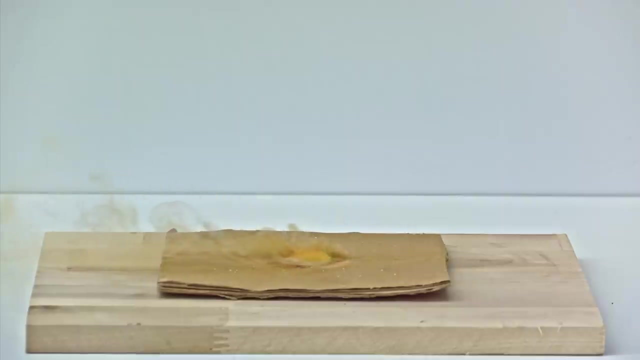 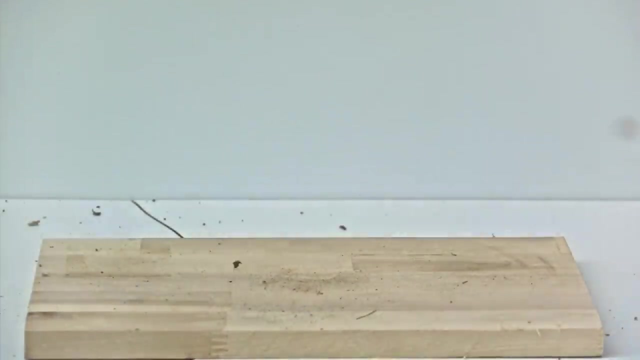 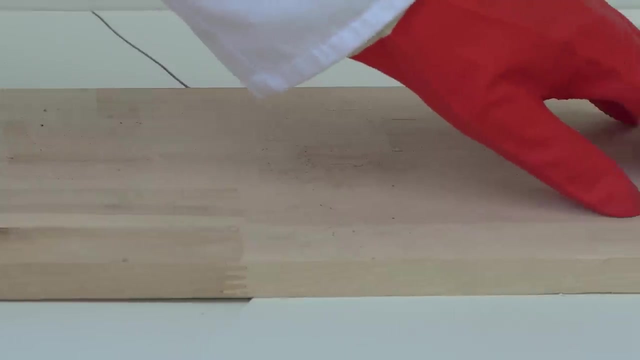 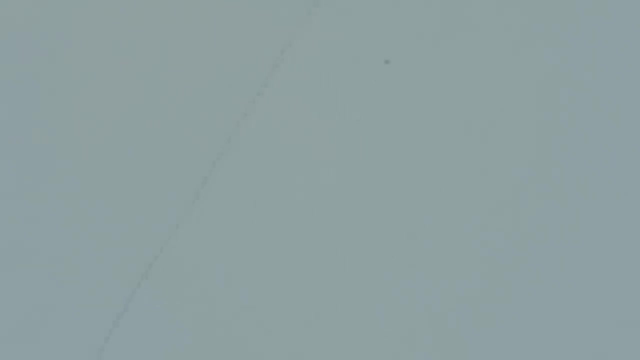 They formed when I carried out this reaction on cardboard and a wooden backing. So what do you think? Let me know in the comments. Bye, Bye, Bye, Bye For such a massive object like a brick. I took a teaspoon of decaborane and added a. 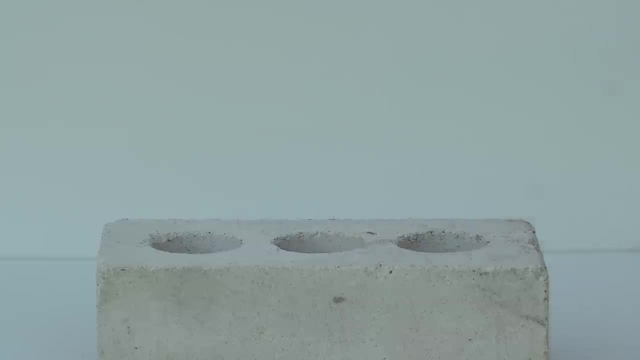 couple dozen drops of nitric acid to it. So what do you think? Do you like it? Let me know in the comments. Bye, Bye, Bye, Bye, Bye, See You, but with another topic. Bye, Bye, See you again. 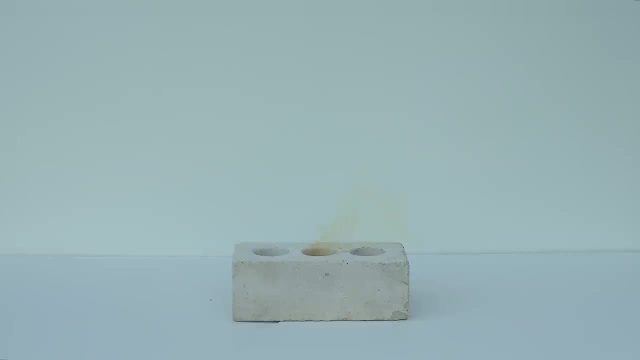 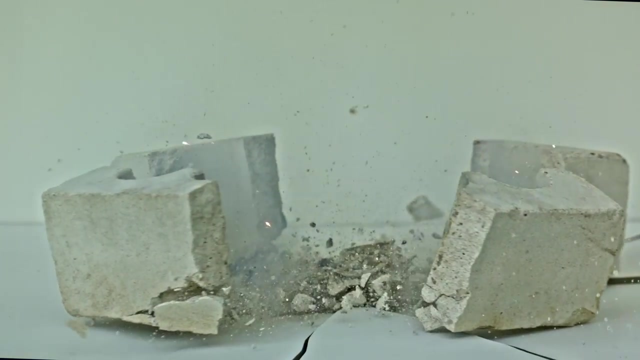 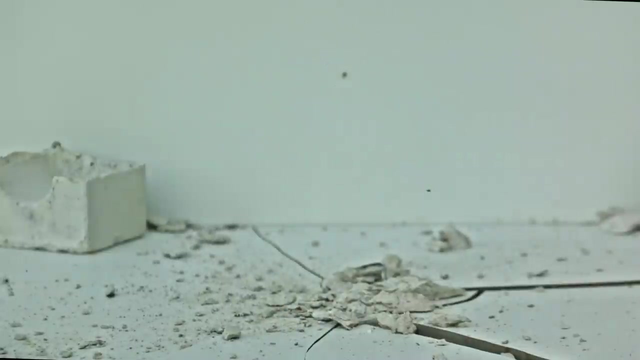 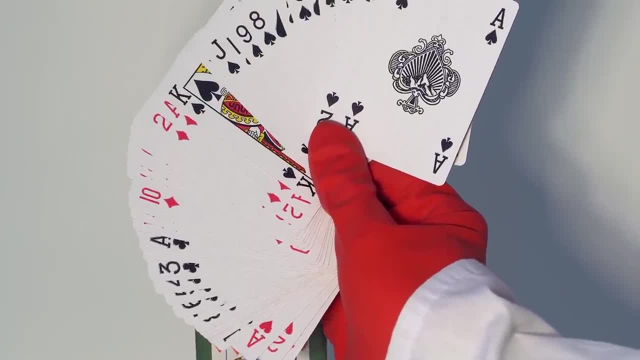 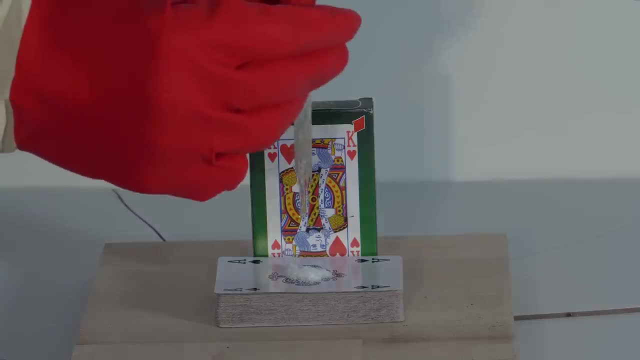 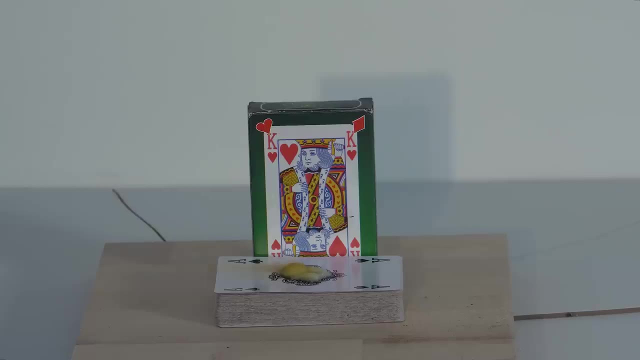 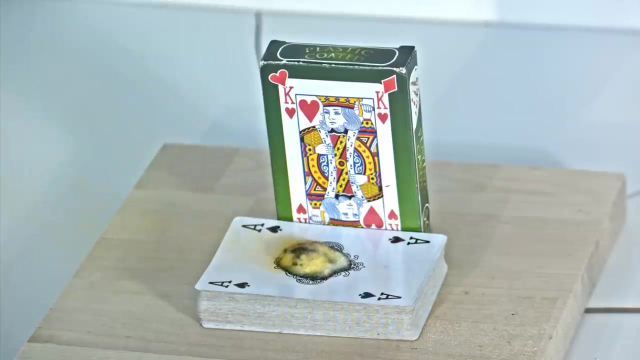 Okay, let's switch it up a bit. Have you ever seen a card trick involving chemistry? Pick any card. Let's say you chose the Ace of Spades. I'll make it disappear using some chemical magic. Let's try to understand the secret of this card trick using slow motion. 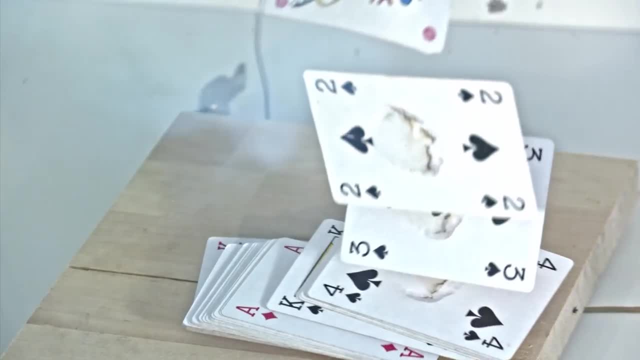 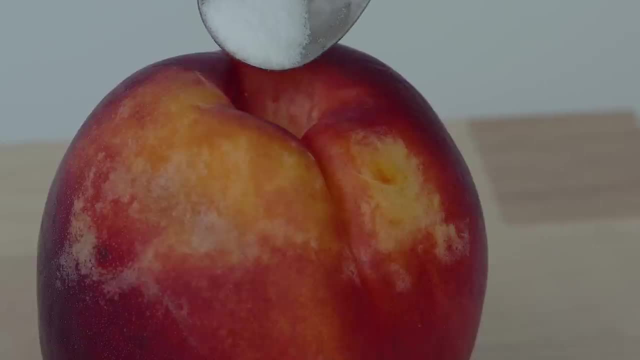 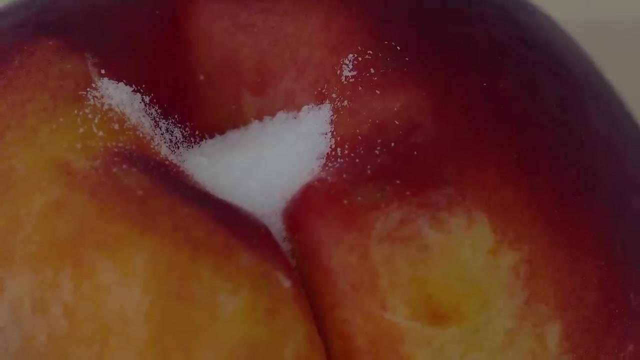 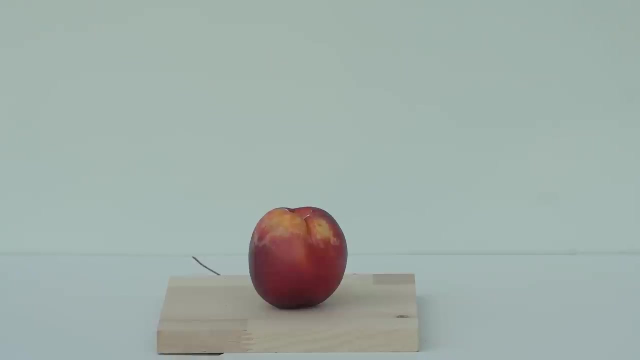 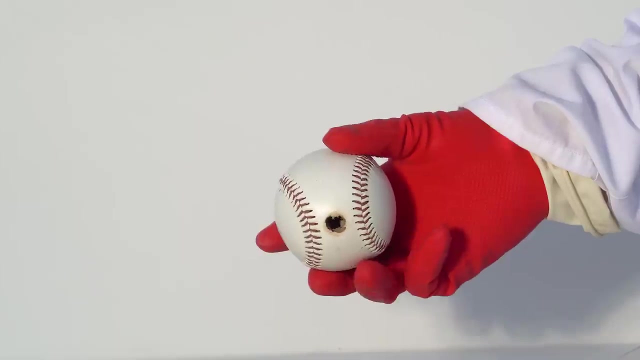 If you know the answer to this card trick, tell us about in the comments. Now let's add a pitch to our reaction. This is an ordinary baseball, and if you don't know what's inside it, then let's find out. To find out, I drilled a small hole in it.